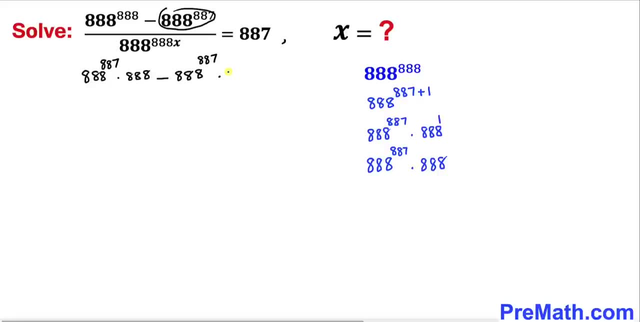 887 times 1.. It doesn't make any difference. Divided by 888 power, 888 x equals to: on the right hand side, This could be written as 887.. And now we can see that 888 power, 887 and same thing. 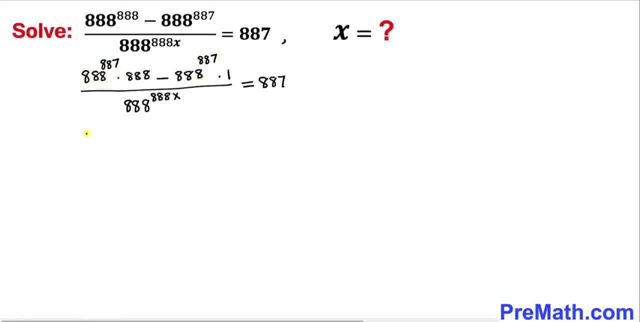 over here common, So therefore we are going to factor them out. I am going to factor them out: So this is 888 power 888 x equals to 888.. And then I am going to write 888 power 887 and then times. we are left with 888 minus 1 divided by 888 power: 888 times x equals. 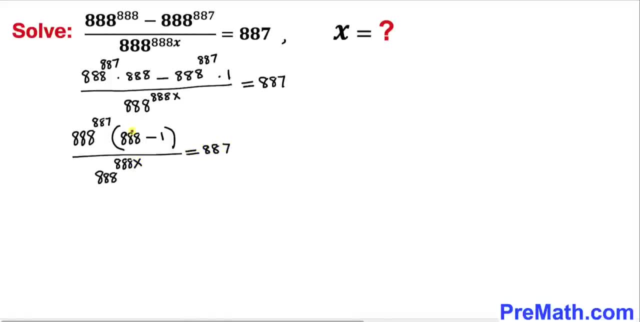 to 887 on the right hand side. Now we can see inside this parenthesis: 888 minus 1 is going to give us 887, so therefore this equation could be written as 888 power 887 times. this is going to become 887 divided by 888 power, 888 x equal to 887. now let me go ahead and multiply. 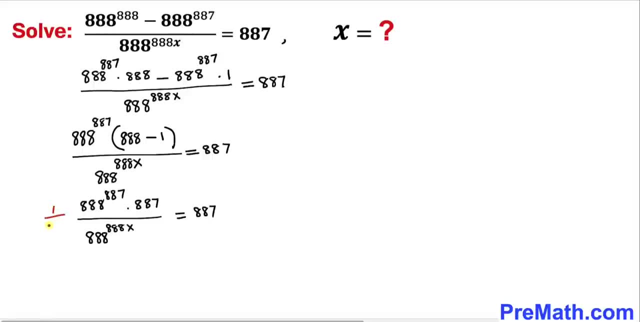 both sides of this equation, by 1 divided by 887 on this side and 1 divided by 887 on this side as well, and we can see that this 887 and this 887 is gone, and likewise on the other side they are gone as well. so therefore, on the left hand side, we are ended up with 888 power. 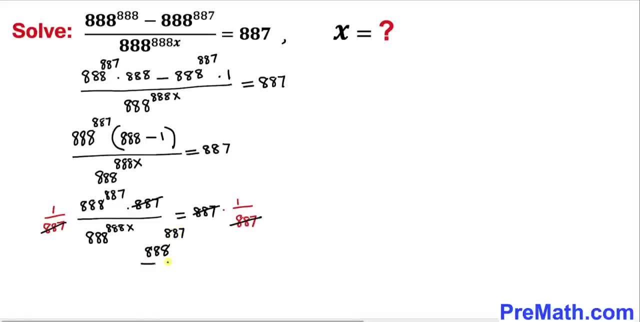 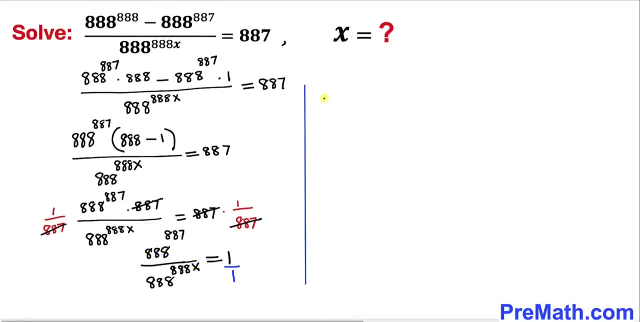 800 887 divided by 888 power 888 x equals to 1. now, on the right hand side, 1 could be written as 1 over 1. this way, we can make it a fraction. let's go ahead and cross multiply, so as a result, we are: